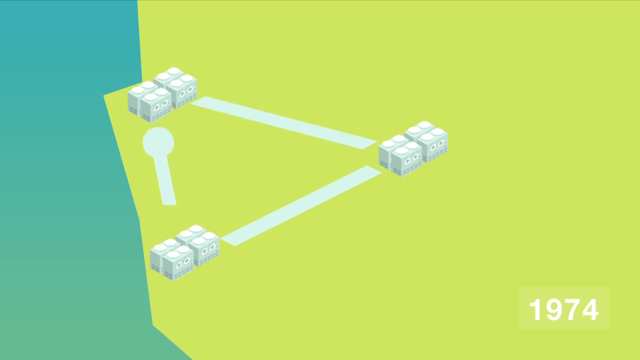 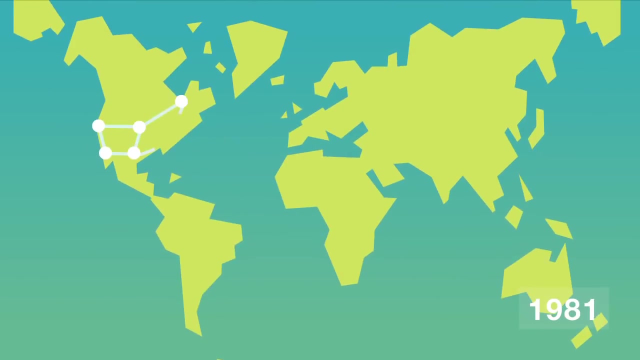 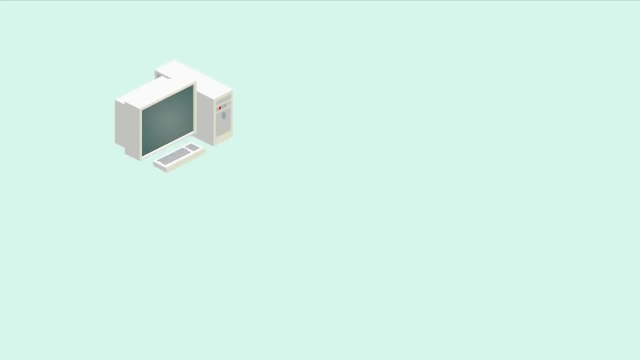 was to let these massive supercomputers talk to each other, And as soon as two computers could send information back and forth, we had a network. The network gradually grew until personal computers emerged in the 1980s. and then it exploded Soon: people were not just talking to each other, but also exchanging money. 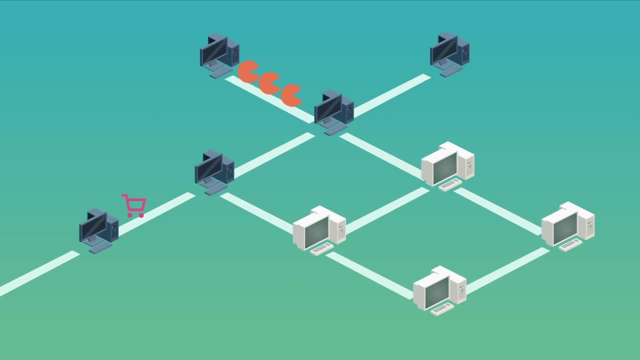 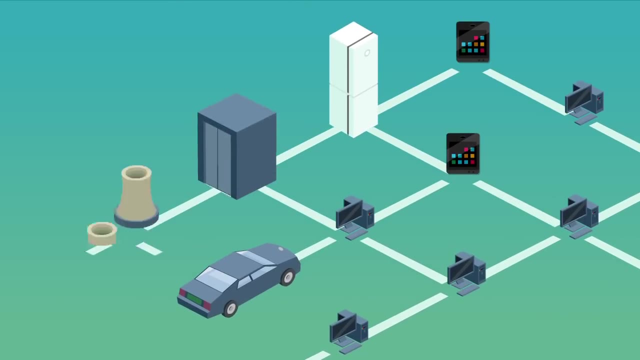 playing games, reading news, shopping and doing everything we associate with the internet. today. Other devices started talking to the network too: Phones and cars, and refrigerators, and elevators and power stations, And so the internet was a place where people could talk to. 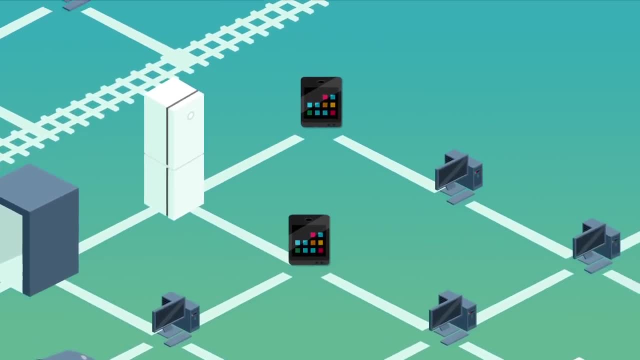 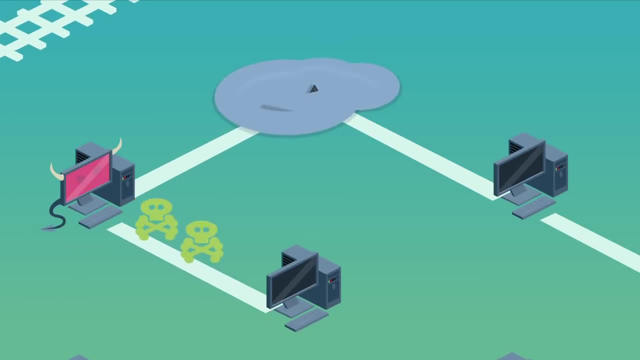 each other. But the ease of all those devices talking to each other came at a price Security. One computer could send another instructions to delete everything on it or take it over. We call these viruses and malware. Or one person could steal another's identity by guessing. 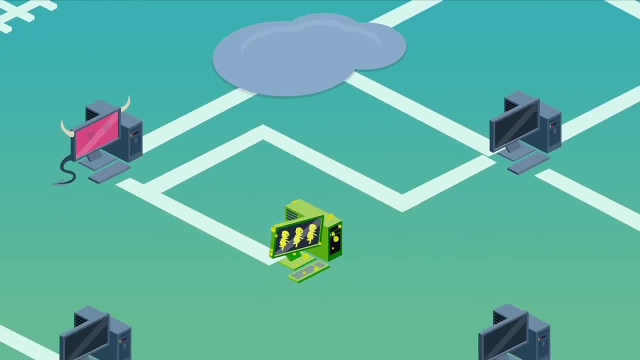 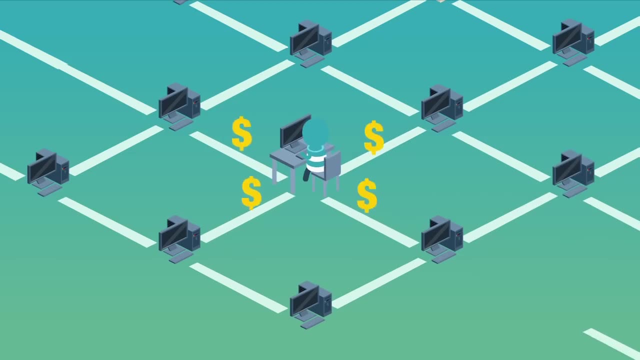 cracking or extracting a password. Vulnerabilities such as these will never completely go away, because they're built into the internet's very architecture. Criminals use them to steal billions of dollars, Governments use them for surveillance, And so the internet is built. 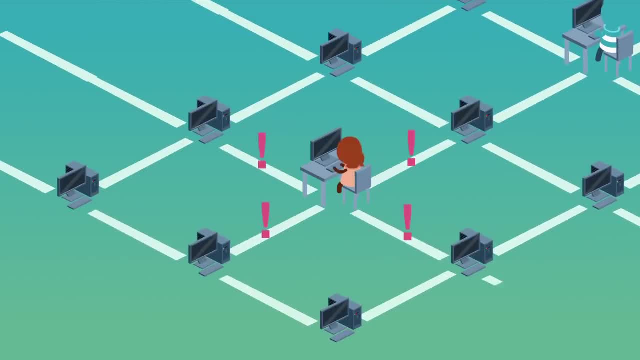 into the internet's very architecture. Criminals use them to steal billions of dollars. Governments use them for surveillance. Criminals use them to steal billions of dollars. Governments use them to steal billions of dollars. Criminals use them for surveillance And hackivists use. 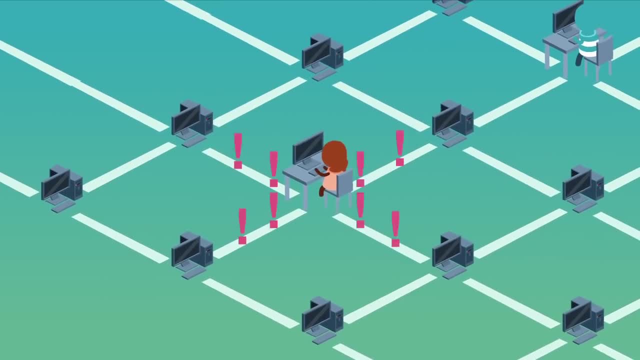 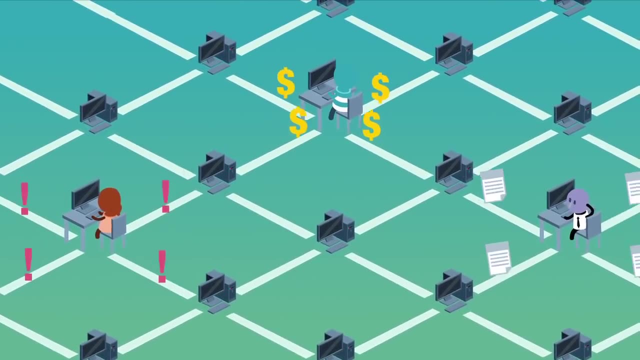 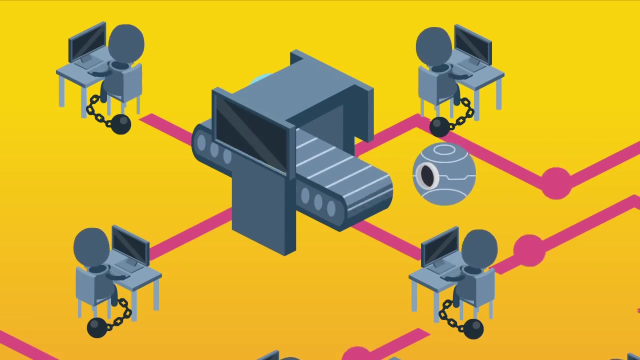 them to further their political goals. Between 2004 and 2013,, over 1 billion records of personal information were stolen or leaked through data breaches of major organizations. As a thought experiment, let's imagine what a perfectly secure internet might look like. 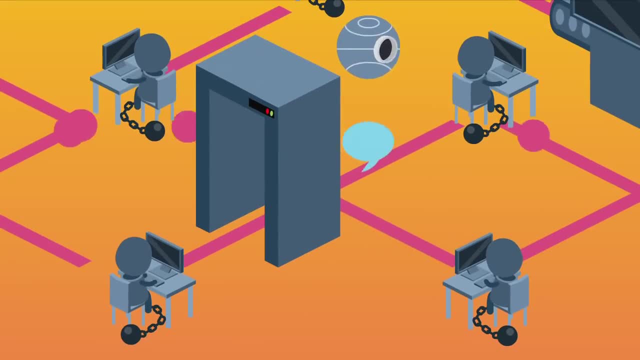 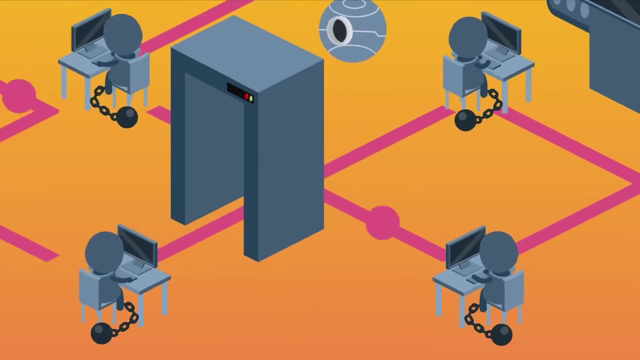 Users would not be allowed to download or install anything onto their computers. All internet traffic would be monitored and regulated by bots and humans, massively limiting the number of websites you could visit. In order to log on to a website, you'd have to type in a 100-character password: submit. a genetic sample and whistle a tune. The servers that hold data would be kept in heavily armed fortresses On the moon. And even with all these safeguards in place, some clever hacker would almost certainly still find a way in. The good news is, even with our flawed internet, there are simple things you can do to protect. 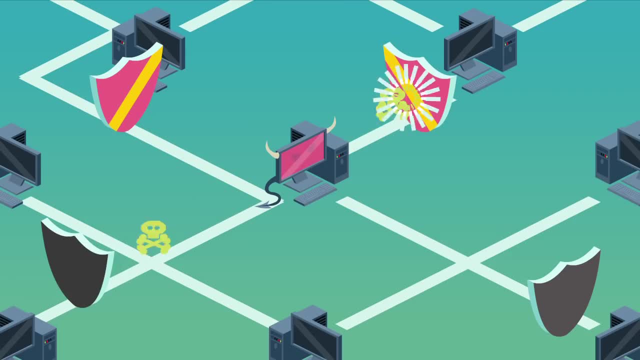 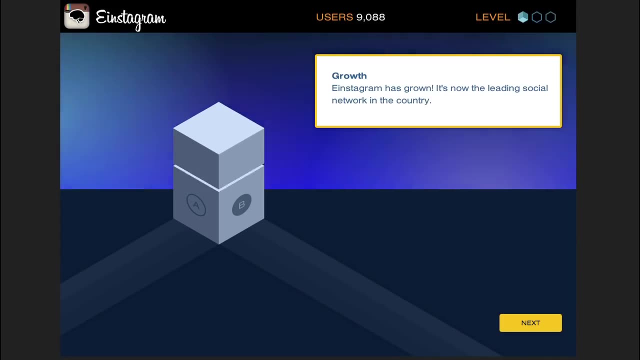 yourself. There are a lot of people committed to making the internet more secure. In Nova's Cyber Security Lab, you'll play as one of these people, protecting a company that's the target of increasingly sophisticated cyber attacks. You must continuously strengthen your defenses to thwart these attackers. 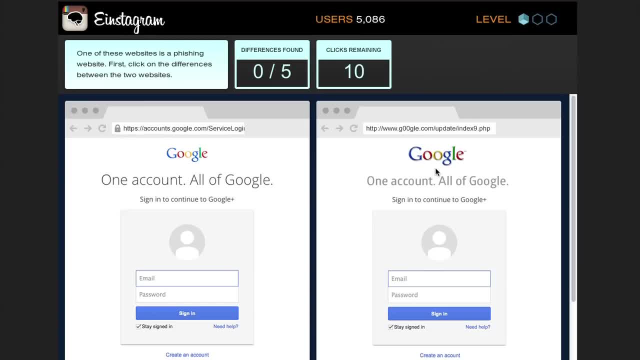 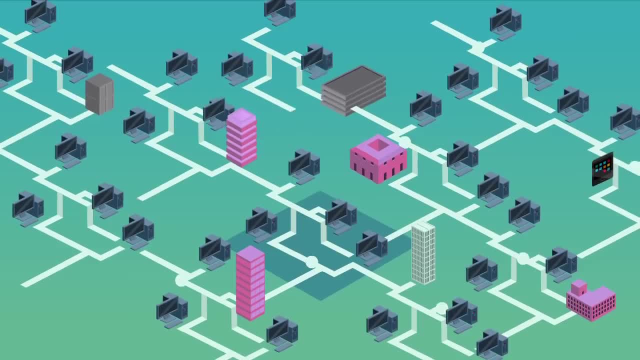 You'll do this by completing challenges that will give you basic coding abilities, help you spot scams designed to trick you into giving up your secrets, and teach you how passwords are cracked and strengthened. The house that is the internet may be built on a shaky foundation, but it's been a home. 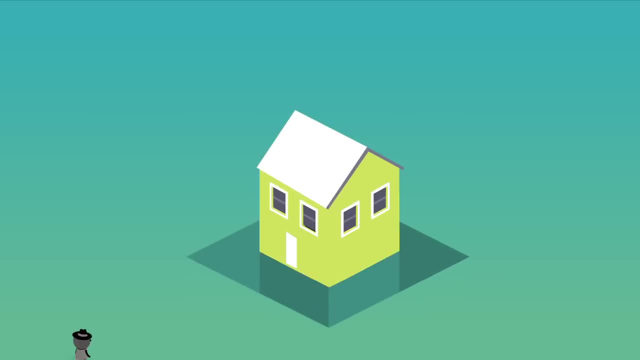 to innovation, Innovation and an unprecedented free exchange of ideas. It's up to us to make it livable in spite of its flaws. 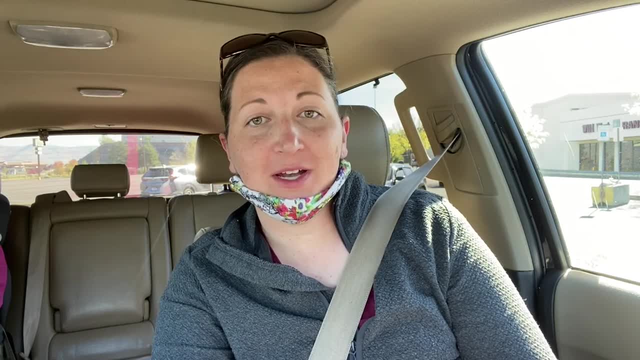 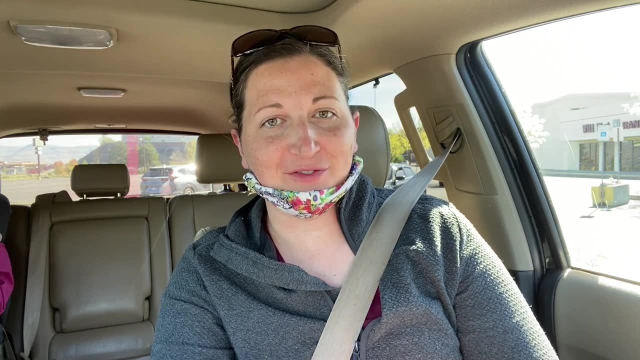 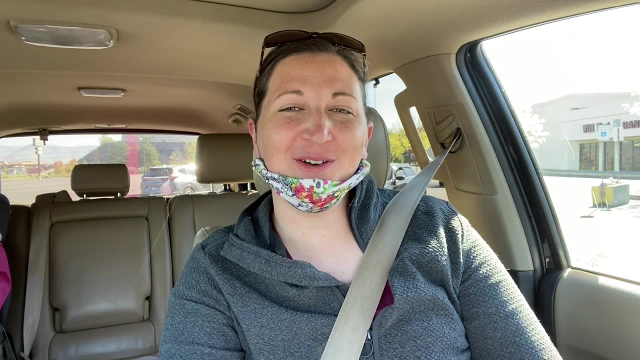 Hi, there it's Stephanie from Mommy Standard Time, where we save minutes and savor moments. Today's Friday, which means we either fail at something or we have some $5 fun, And if you caught my last week's video, which was a big fail, you'll know it's probably time for some fun. 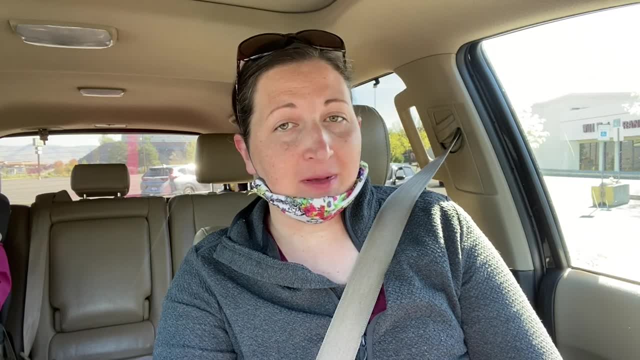 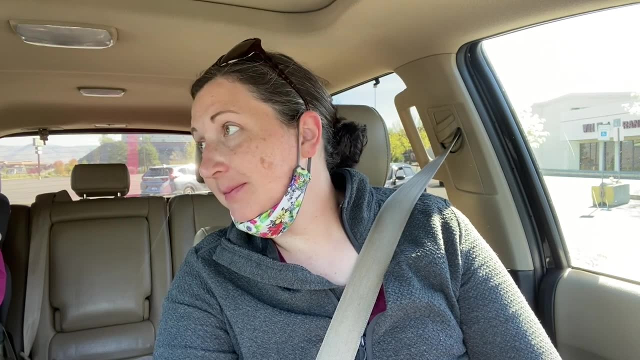 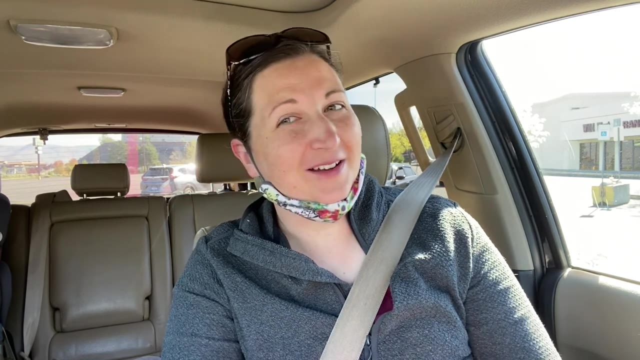 So I have been working outside all week like big outdoor chores. It's springtime, there's just a lot to do And, frankly, Ladybug is bored, aren't you sis? Are you bored with being outside all the time? Yeah, but not if there's fun. But not if there's fun. So I thought that it would be fun to go. 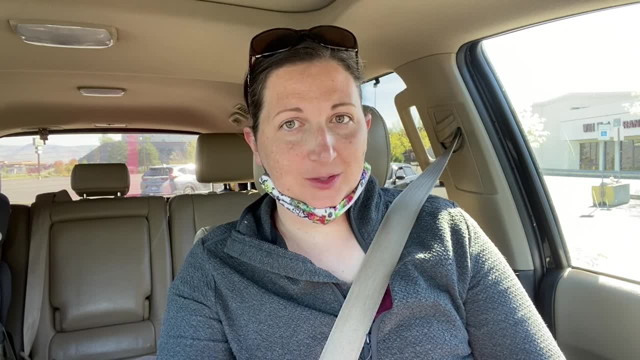 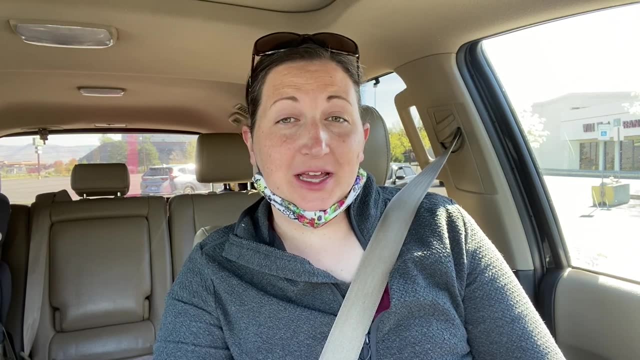 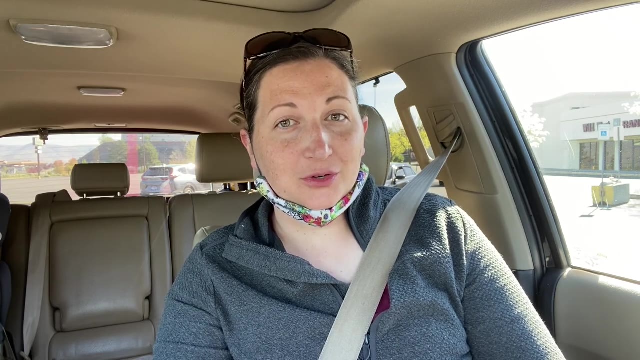 ahead and create a solar oven. Ladybug's been watching Emily's Wonder Lab on Netflix- Awesome show if you have not watched it, But they. yesterday she watched the episode where they make solar ovens And I thought, well, how fun. So we're going to go to the dollar store. I am at. my local dollar store. I'm going to go to the dollar store. I'm going to go to the dollar store Where they have a freezer section and they have more food, but they don't necessarily have a lot of the other things, And so fingers crossed that we not only get the food we need for the solar. 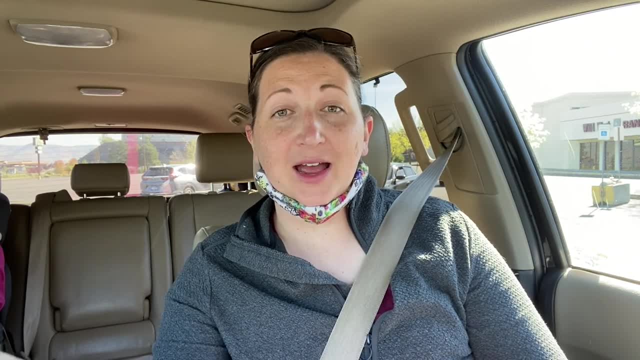 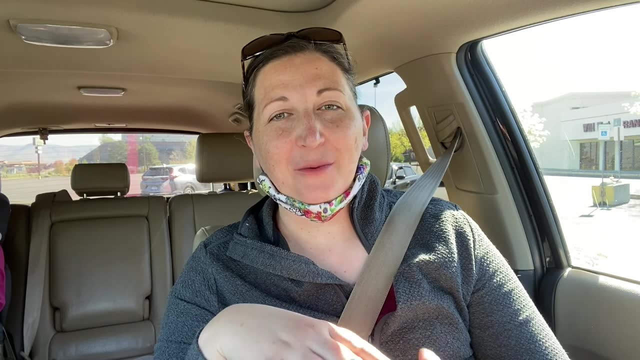 oven, but also the materials we need to build the oven And, as always, this will be $5.. We're actually going to do it two different ways, So I'm spending $10 today, but I wanted to show you that you can either do an all-in solar cooking activity.